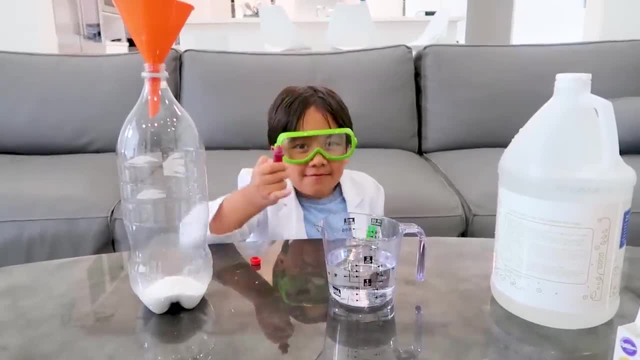 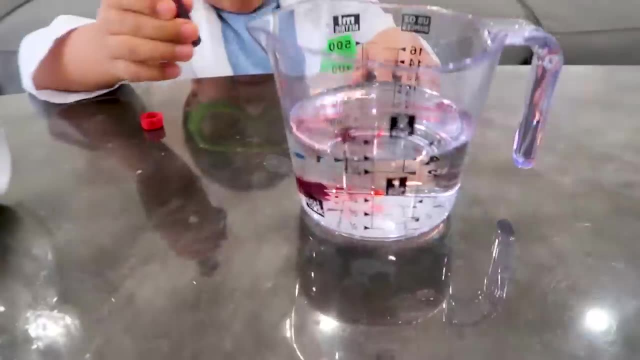 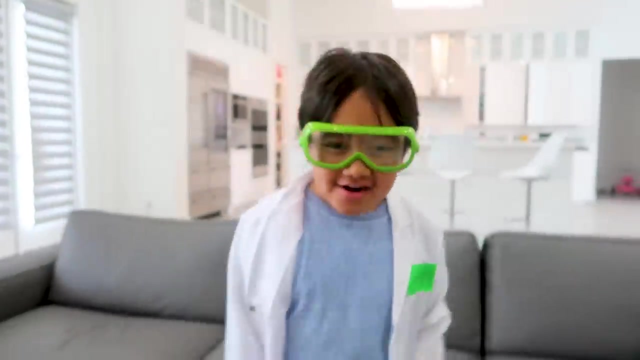 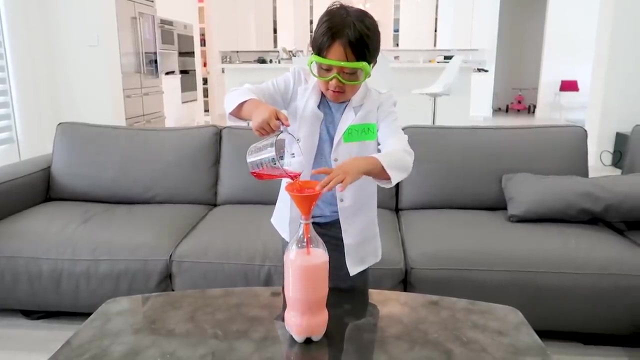 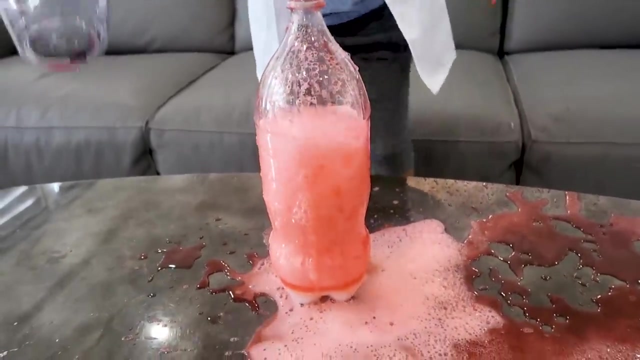 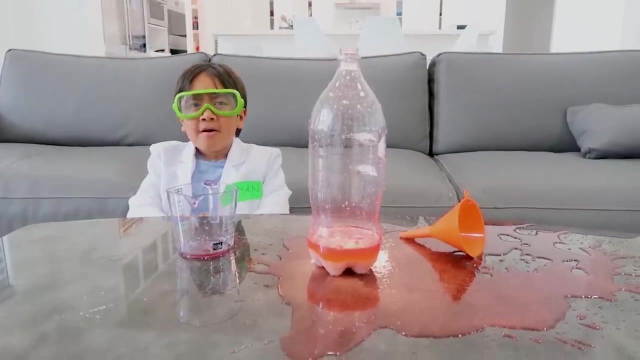 Okay, next you're going to put your food coloring into your vinegar, and I choose red A little bit more. Okay, guys, get ready for an experiment. Remember, ask your parents for help. Whoa, that came out. That was so cool. That was really fun, but I wish it was a volcano. 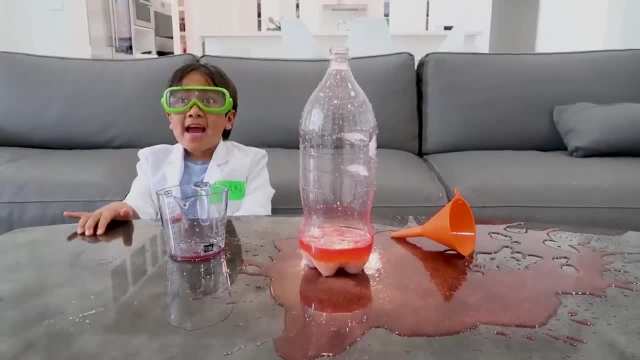 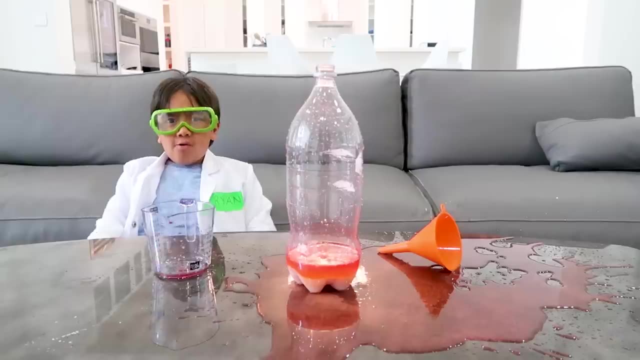 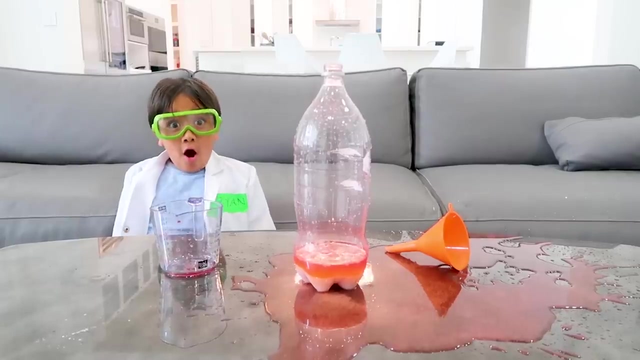 Oh, Peck, Hi, Peck. Gosh Ryan, did you know that you can make a volcano out of paper? What You can? Of course you can. I'll go make one for you. Okay, I'm going to build a Lego robot. It's going to be my best friend. 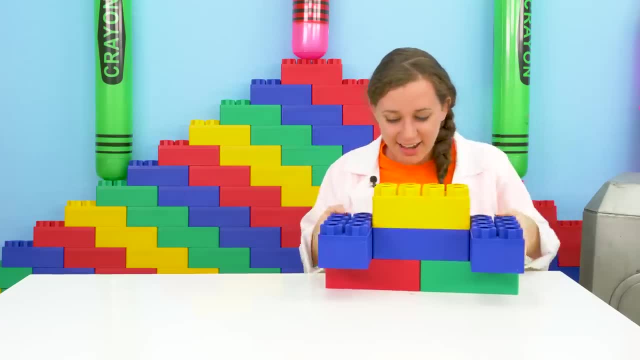 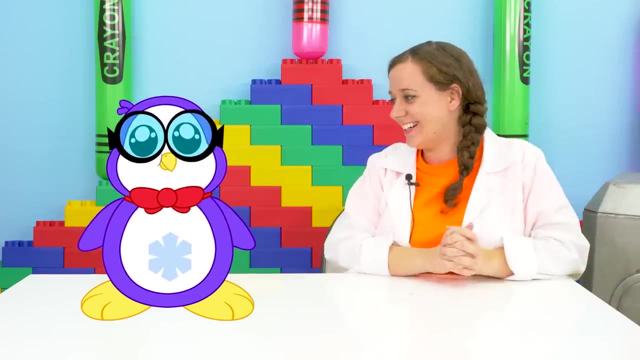 All I need is the last piece for the head, and oh, it's so cute. Whoa, whoa, Uh-huh Peck. What are you doing here? We got a new science experiment for Ryan. It's going to be a giant volcano. 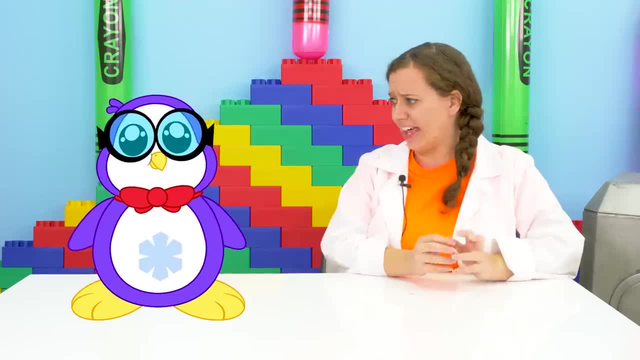 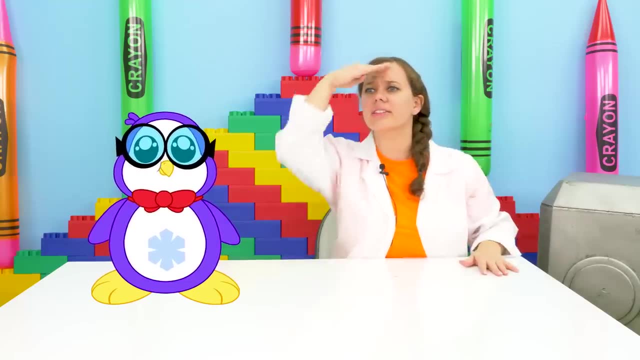 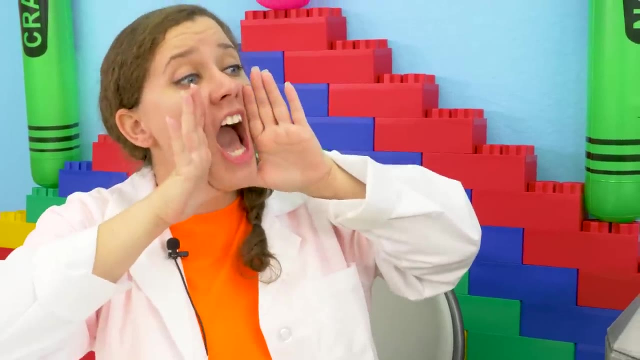 A giant volcano. Well, what do we need for that? First thing we will need is a giant box. A giant box. There's definitely one around here, Let's see. Oh, over there by Combo. Hey, Combo, pass the big box. 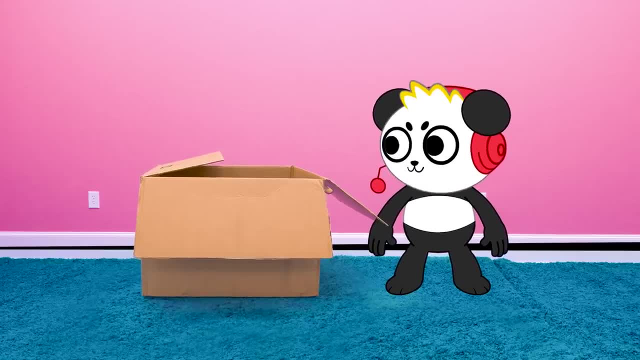 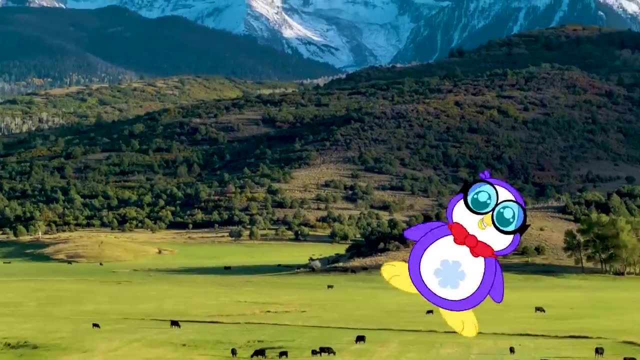 Huh, Oh, this box, You got it Bree. Hi-yah, I'm a little teacup shark. Whoa, Ha, ha, ha, Yeah, Whoa, Whoa, Whoa, Yeah, perfect. 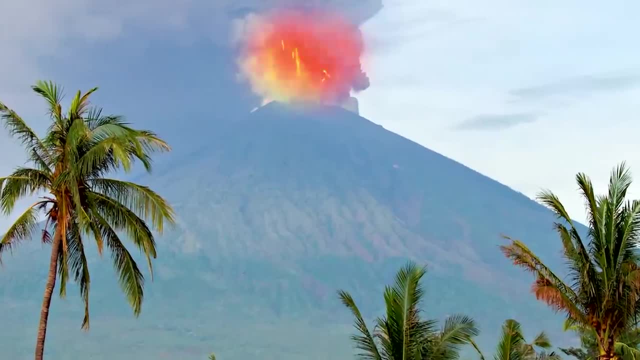 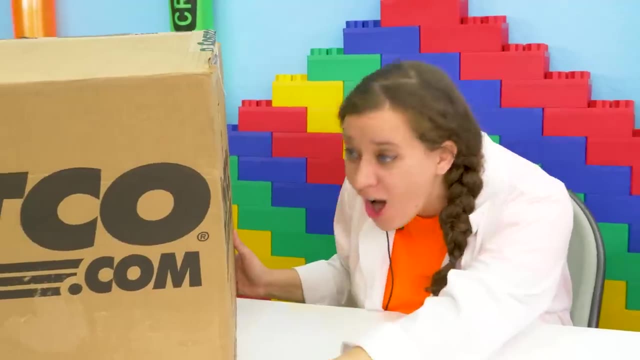 This place doesn't seem too familiar. Huh, What's that? Looks like there's a volcano nearby. Let's go investigate. Whoa, This box is huge and it is going to be the perfect base for our volcano, Don't you think, Peck? 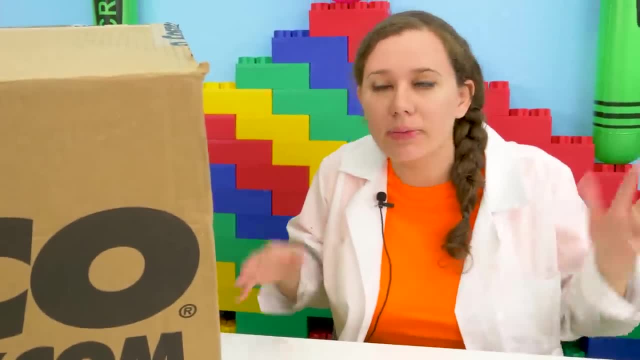 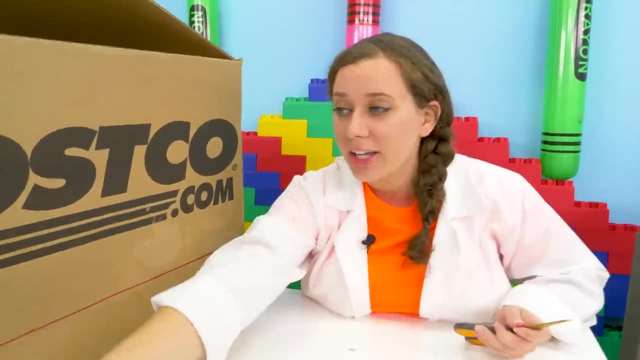 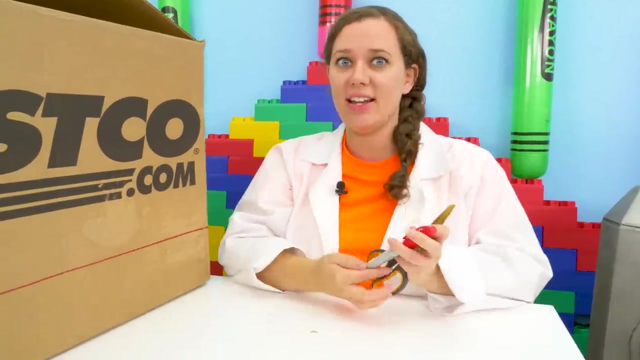 Peck. Where did Peck go? Oh well, let's get started. The first thing we need to do is cut this box down, So I finished marking my line Where we need to cut. it's about four inches high, which I think is going to be a good height to keep all the lava inside. 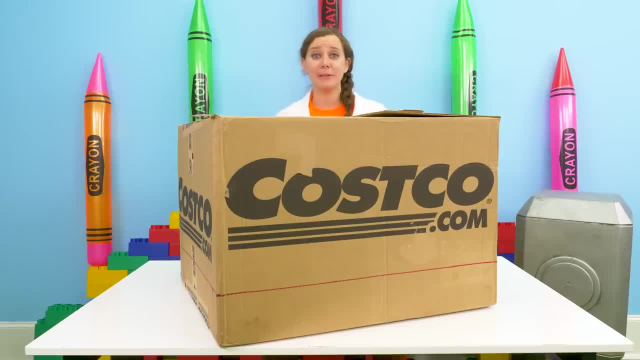 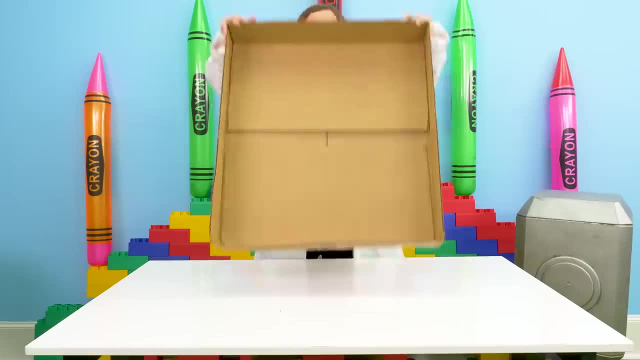 So now all we need to do is cut, And once we cut the box, it should look like: Oh and there it is. That is the perfect size for our base. Look how big it is. Now, to make sure that our base is good and strong, we're going to use duct tape. 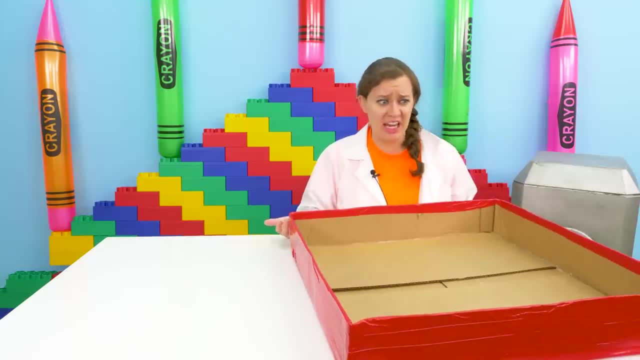 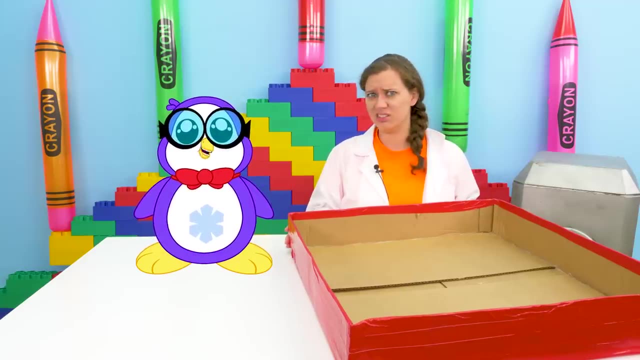 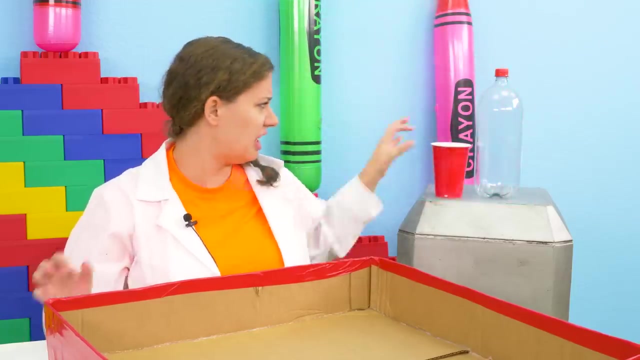 Well, the box looks great, but how do I build a volcano Incoming? Oh Peck, there you are. Huh, I just got back from gathering research data. First, we're going to need These: A bottle and a cup. 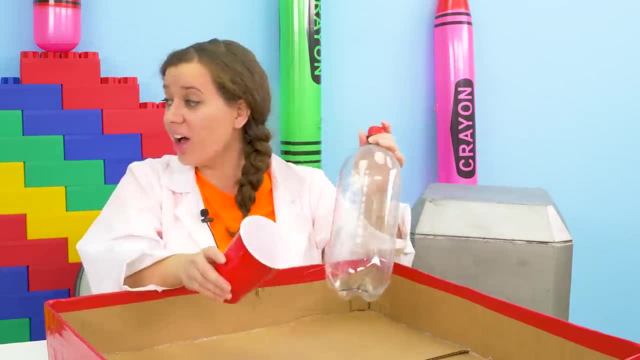 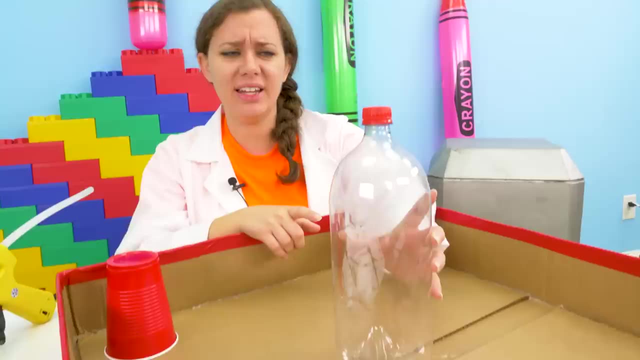 I think we can use this for the center of our volcano Precisely So. this bottle is going to be perfect to put all of our ingredients in for the lava, But I think it's a little too short. That's why we have this cup. 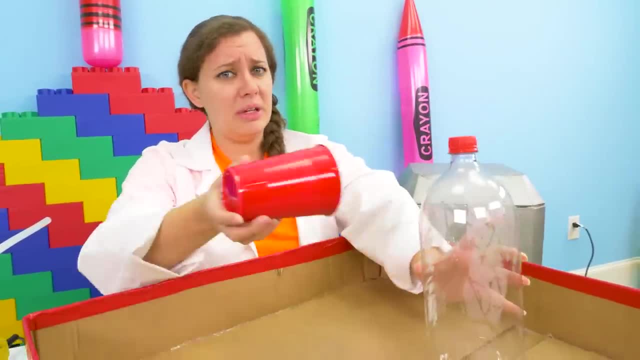 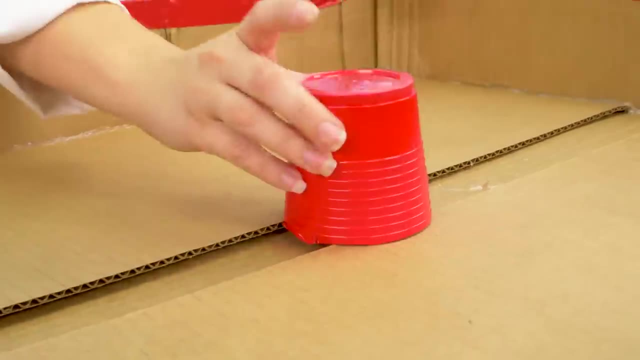 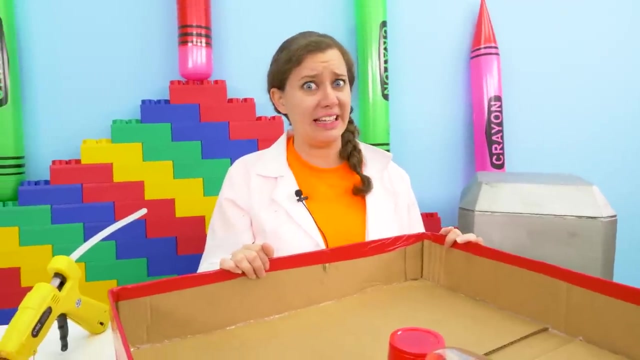 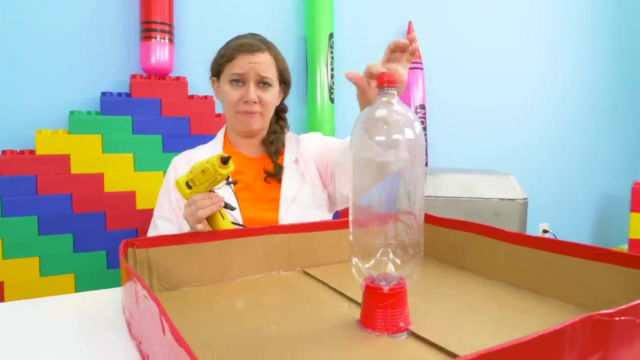 I think that might be a little too tall. We can work on this. Oh Oh, that is the perfect height. Uh, maybe we should glue it in place. Okay, just a little bit more glue, And I think that should do it. 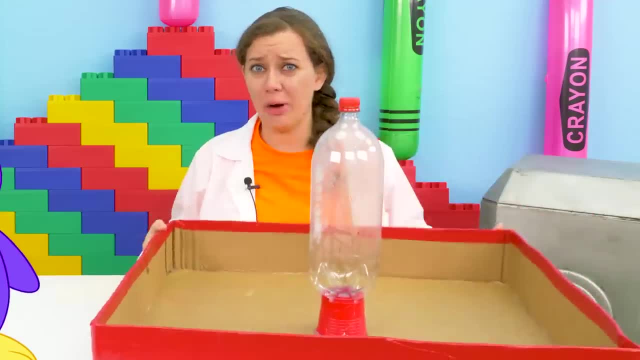 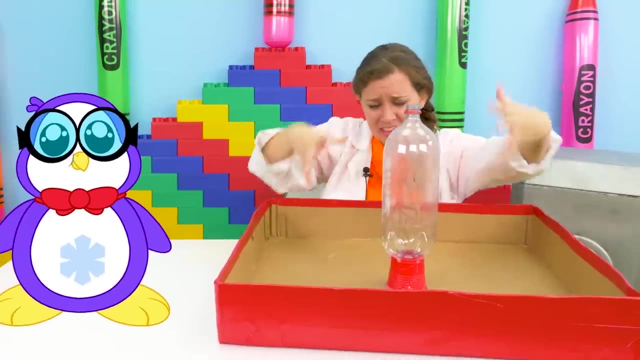 I don't think it's going anywhere. Okay, our bottle's not going anywhere, But we don't need this cap. It doesn't really look like a volcano. We need something- I don't know what. We have to build a body. 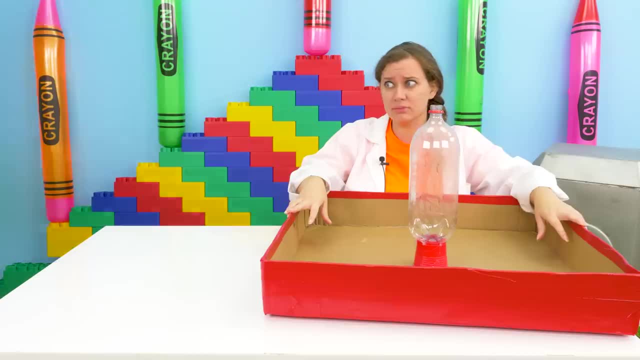 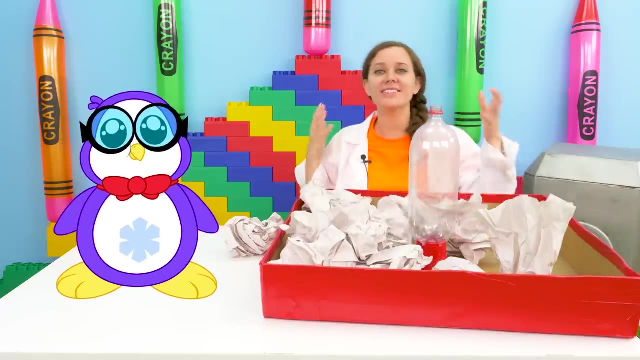 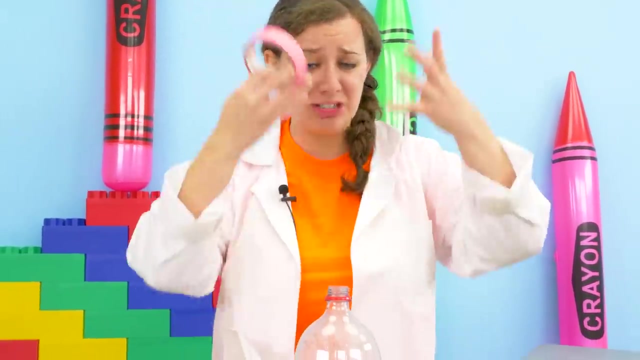 Hey, I know what'll work. Okay, Trash Paper- That's a great idea. So we're making the shape of our volcano. It's kind of a mess right now, So we're going to use tape to hold all of this together. 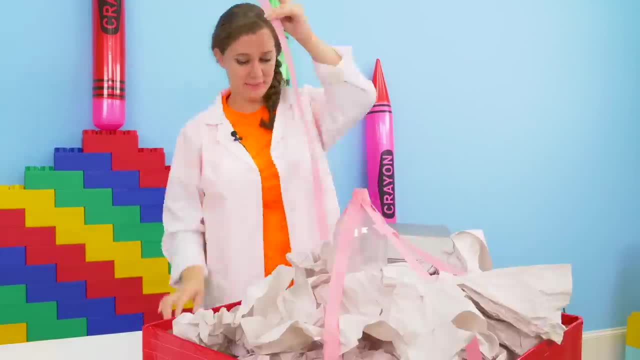 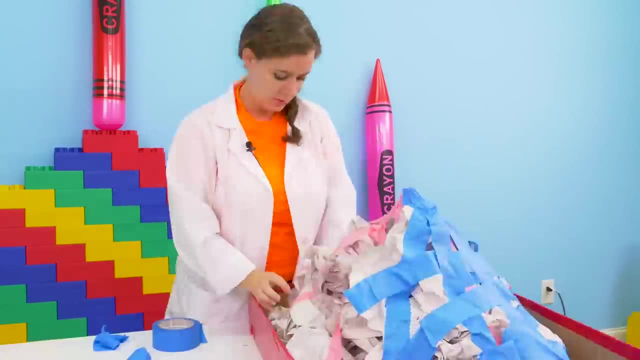 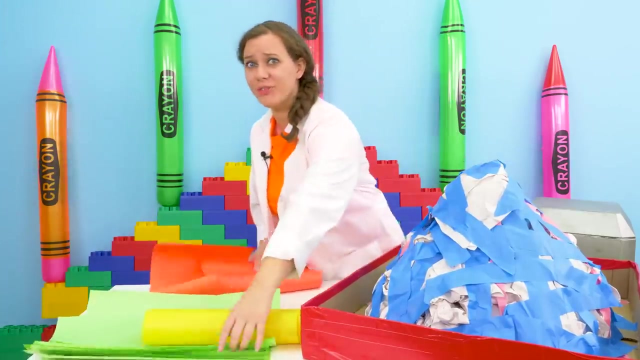 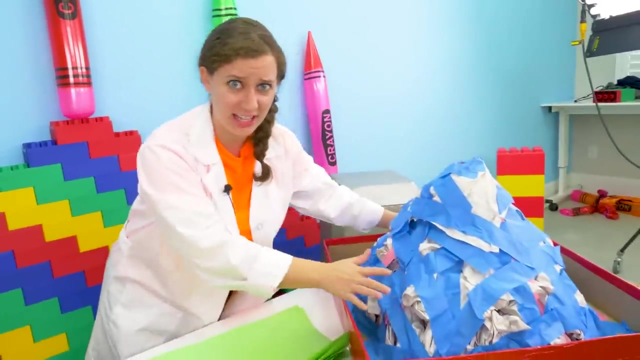 Now to form the body of the volcano with some tape, And then we're going to add some more of this, More paper. Oh wow, Peck, you found a lot of paper. This is going to be perfect. So the first thing that we need to do to start paper machining this giant volcano is: we need 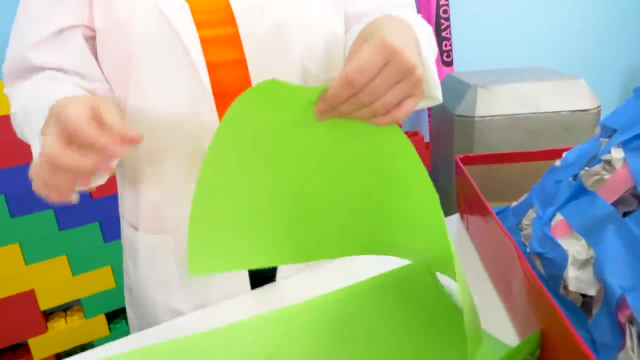 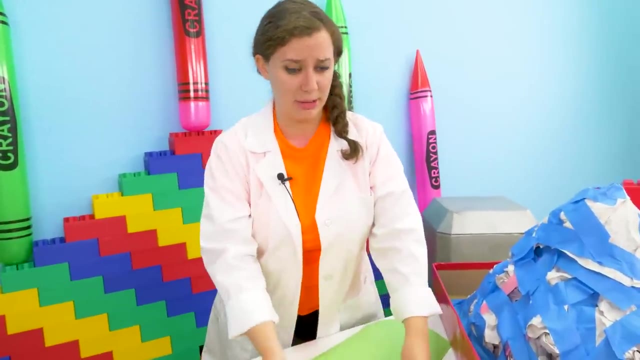 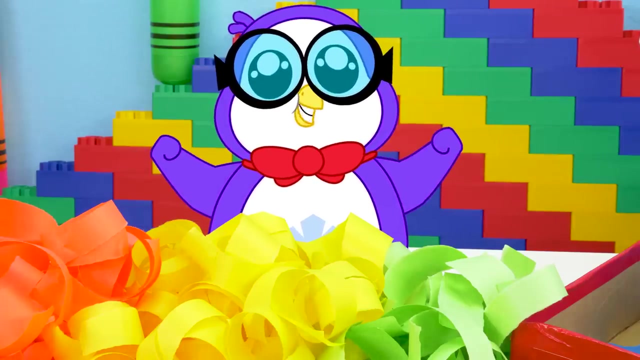 to take all of this paper and tear it into pieces that we can actually use, So something about like that. But we're going to need a lot. This guy is very big. So, Yes, Yeah, yeah, this ought to do the trick. grip the paper, whoa peck. great job. this is a lot of paper. 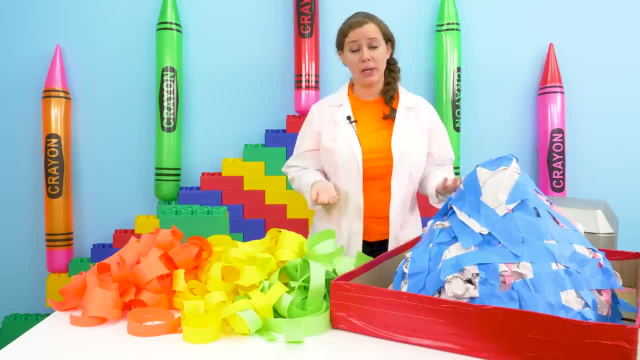 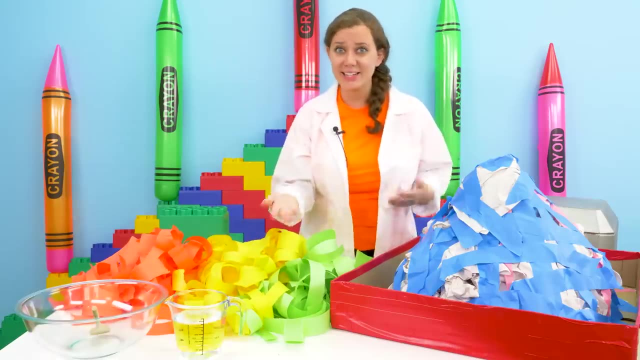 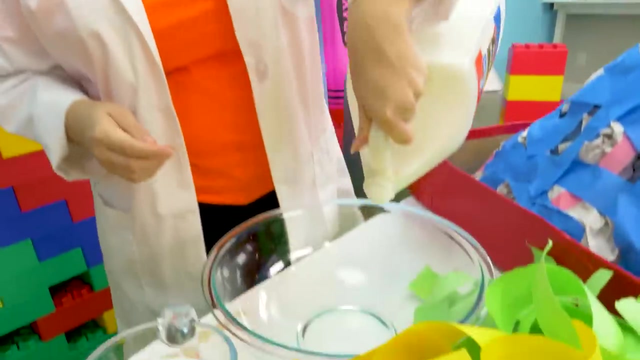 what else do we need? uh well, to make paper mache, we need paper, which we already have, and then we need a bowl, some water and, the most important part, glue. so this glue is way too thick. so the first thing we're going to do is add glue. then we're going to 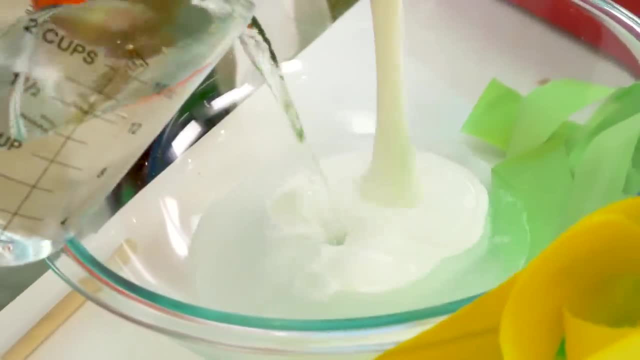 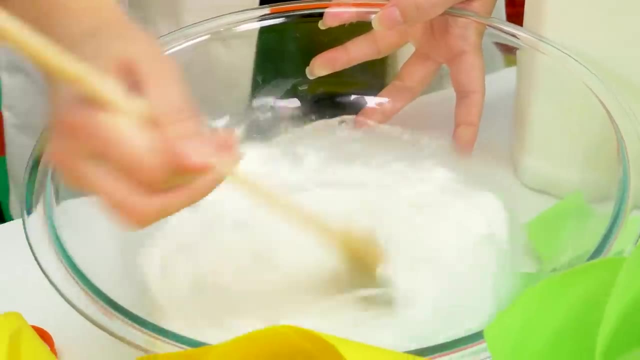 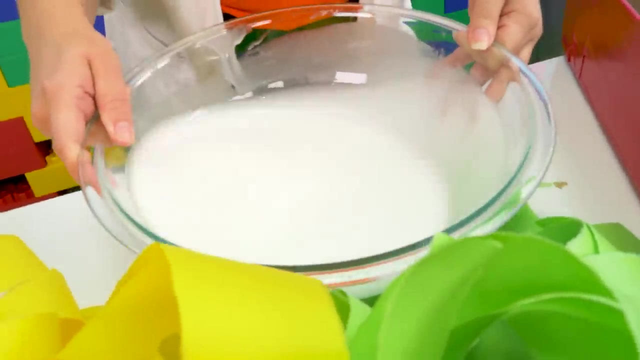 add water and stir it all together to try to thin it out so we can put it on our paper. now we do is stir or agitate, agitate, agitate, and when you're done, it should look something like this: now we're all ready for the fun part. it's going to be a little messy, so if you're wearing 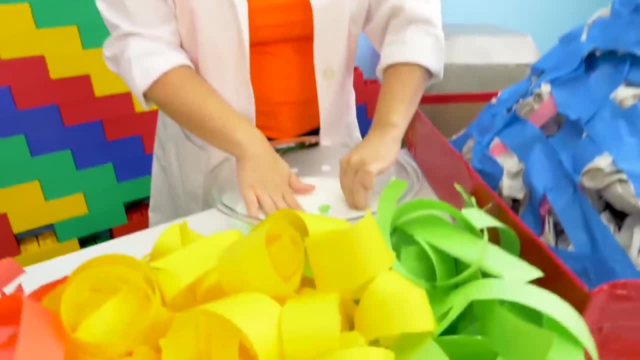 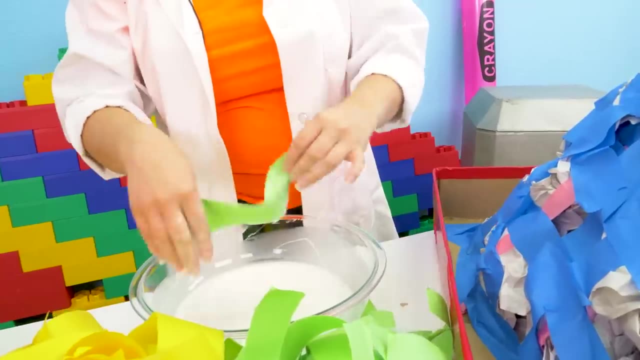 clothes. you're going to want something for the front, so i'm going to put this on for the front sleeves. roll them up. First you dunk it in the glue and then you just clean off all the extra, make sure the paper is good and kind of soft, and then you just 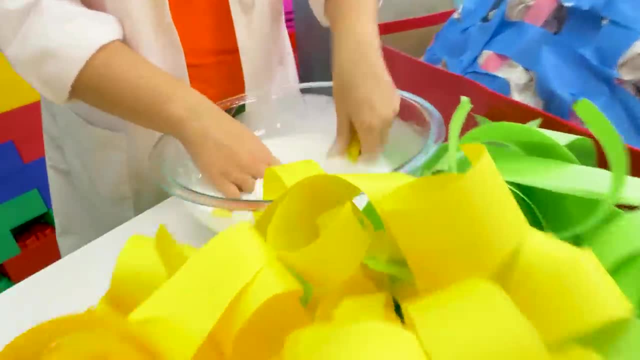 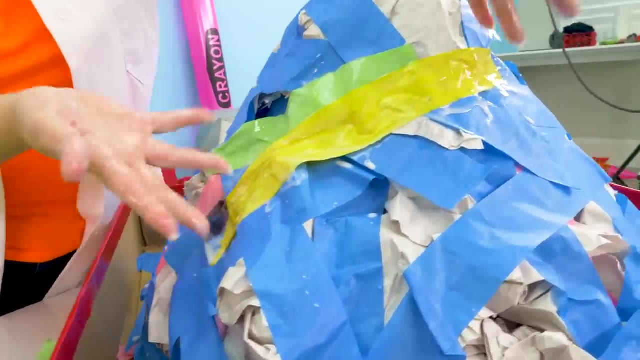 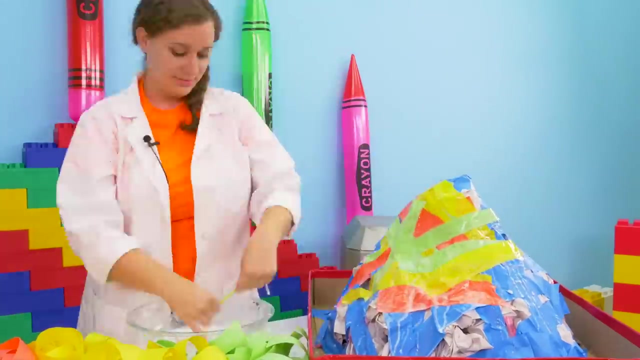 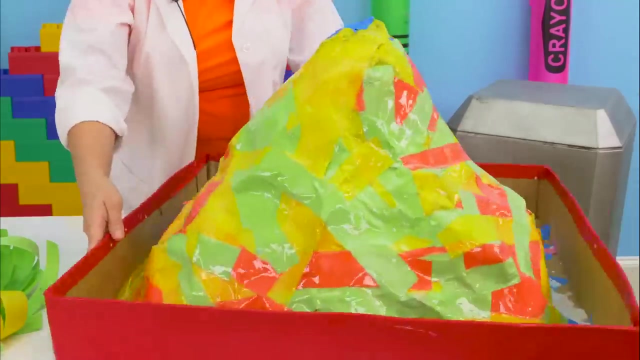 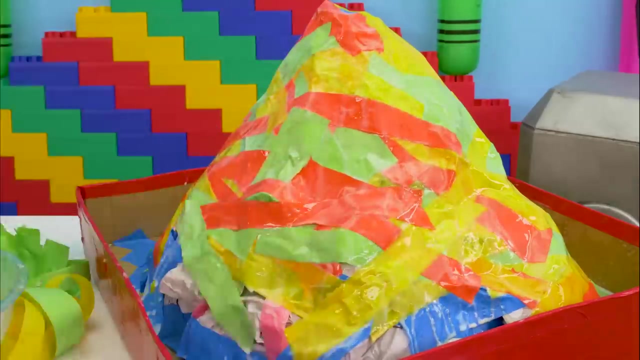 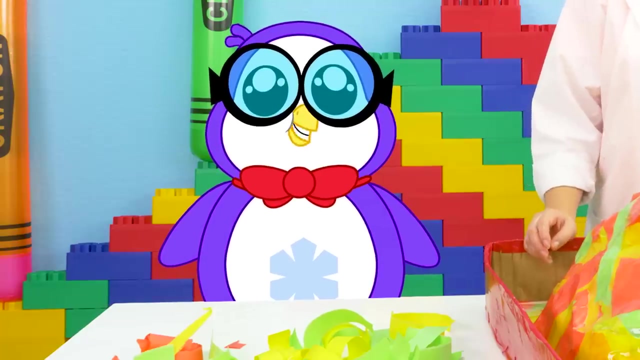 slap it on the volcano- Wow, Slimy. Now the hardest part. we have to wait for this to dry. The volcano will take a while to dry. Let's go wash our hands. Oh yeah, I'm very sticky, so we'll meet back. 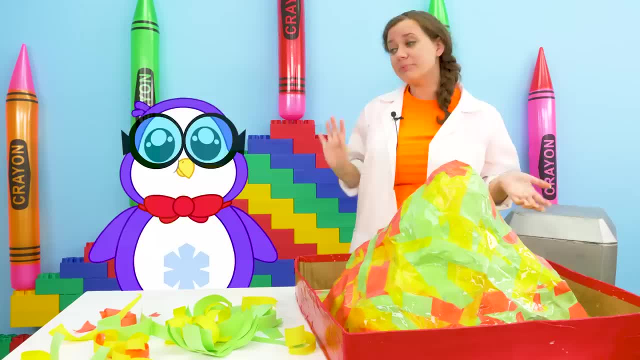 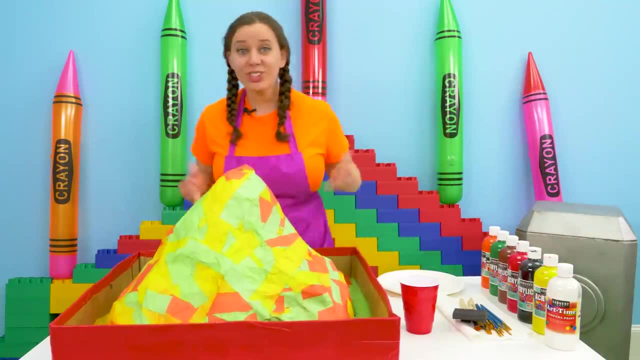 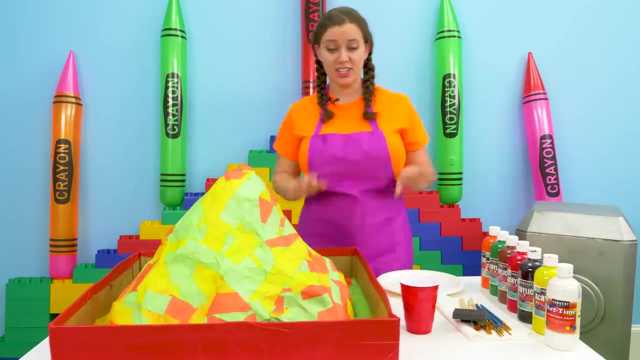 here later. Yep, I'm gonna go gather more research. Bye, Oh shh. One day later, Whoa, it looks so good and it's really dry. let's see. it's definitely hard and sturdy, ready for paint, but where is Peck? Peck, Are you free, Peck? Oh yeah, I'm at a real volcano and, um, I think we need to use a gray paint. 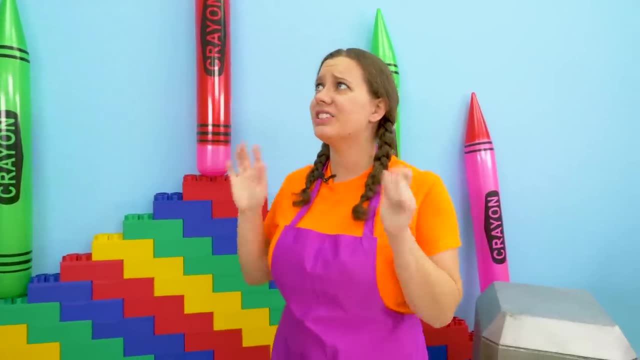 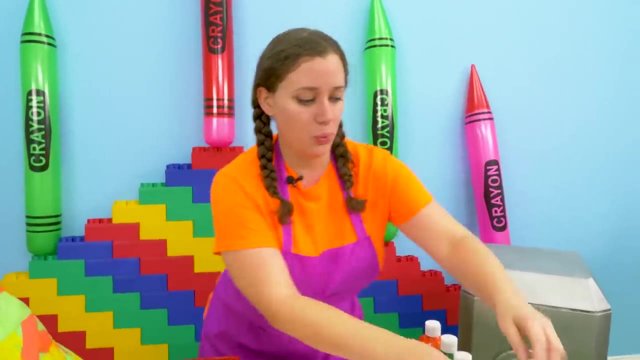 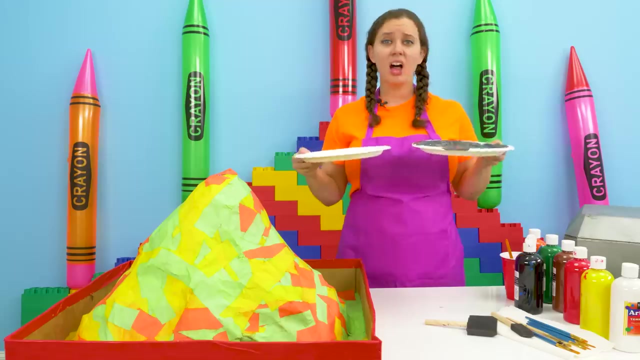 Well, we can definitely make gray Peck, but just make sure you stay safe. okay, be careful. Now, gray, we don't actually have, but we can make it with black and white. All right, Peck, how do these grays look? Oh yeah, I think I know what you're talking about. 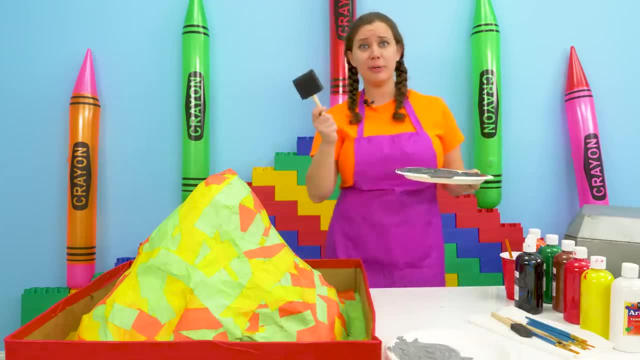 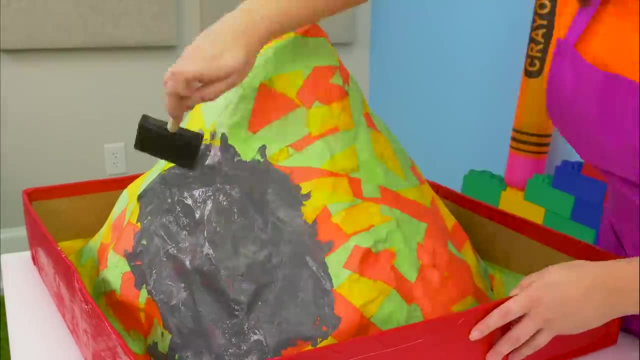 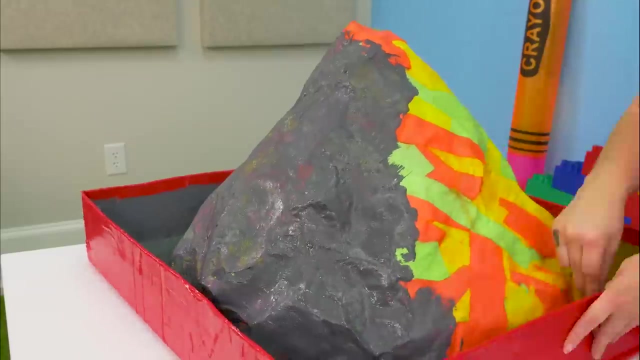 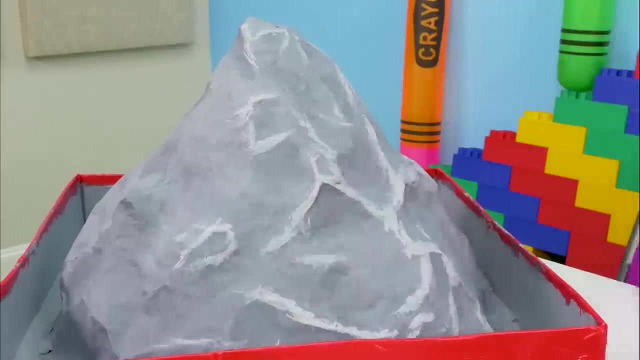 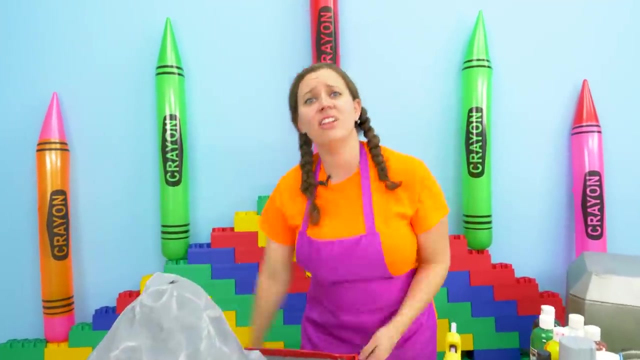 Oh yeah, I think I know what you're talking about. Oh yeah, I think I know what you're talking about. All right, well, it's a big volcano, we're gonna use a big brush and let's get started. All right, we all right. we just finished all of this painting this. 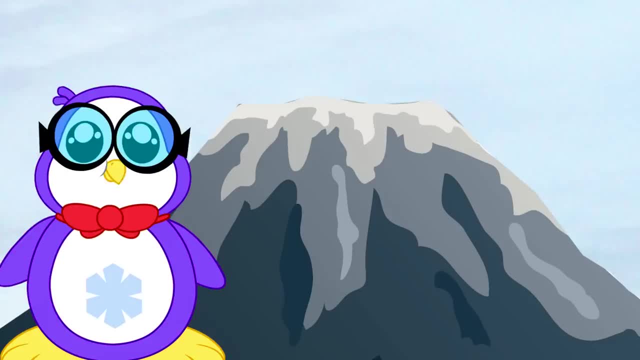 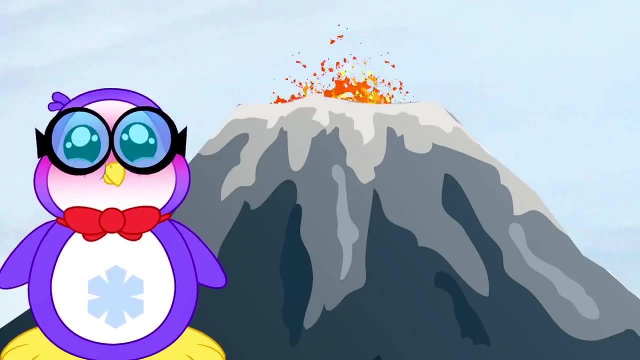 just finished all of this painting. this volcano is huge. it took forever peck. how does it look? it kind of looks just like a mountain. it could use some lava, some lava. oh yeah, awesome lava. i'm gonna head back now. it's getting a little hot over here. 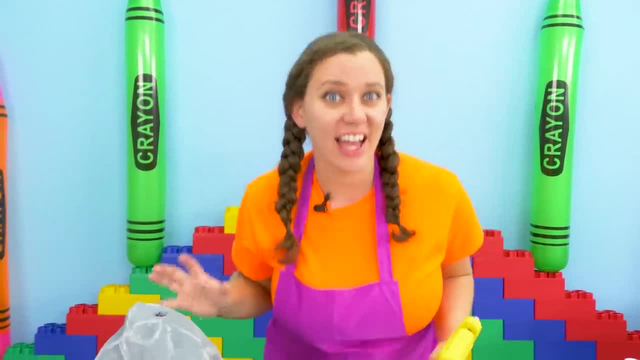 okay. well, we'll see you in a bit peck. now i have a great idea for the lava. what better than hot glue? i mean it kind of looks like lava, right for the lava, what better than hot glue? i mean it kind of looks like lava, right, maybe? 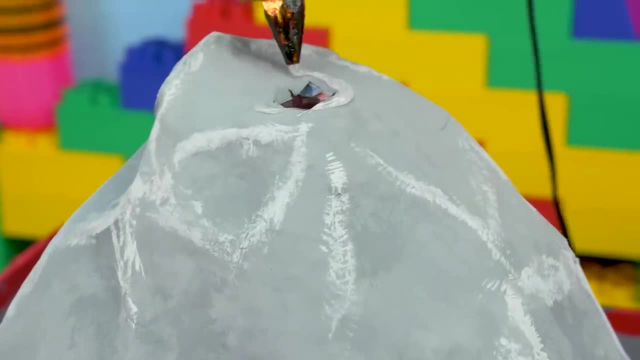 for the lava. what better than hot glue? i mean, it kind of looks like lava, right, maybe? all right, let's see. so we're gonna try to build it up and see if we can get it all right, let's see. so we're gonna try to build it up and see if we can get it. 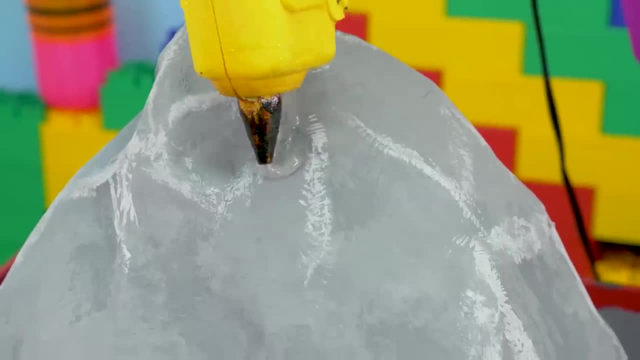 all right, let's see. so we're gonna try to build it up and see if we can get it to look like some, to look like some, to look like some big giant lava trails. big giant lava trails, big giant lava trails. whoa, that looks so cool. 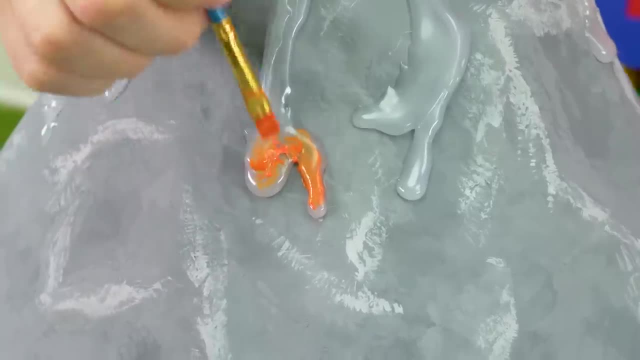 whoa, that looks so cool. whoa, that looks so cool. ah ah, ah. all right, now we're going to use some. all right now, we're going to use some. all right now, we're going to use some orange and some yellow to give this lava. orange and some yellow to give this lava. 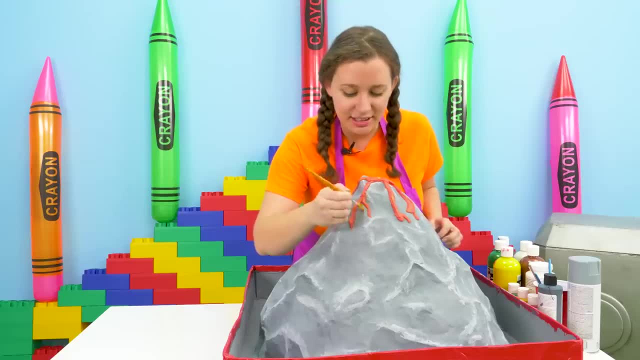 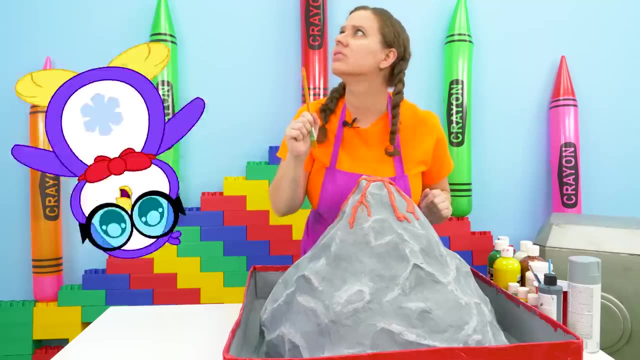 orange and some yellow to give this lava some color, some color, some color. oh, just a little bit more lava paint. oh, just a little bit more lava paint, oh, just a little bit more lava paint. and i think i hear peck, and i think i hear peck. 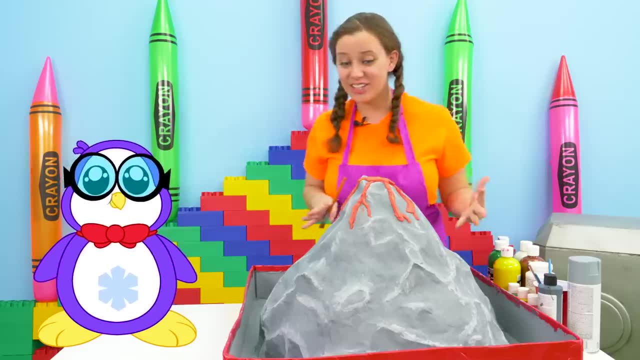 and i think i hear peck made it just in time. oh hi, peck, so we made it just in time. oh hi, peck, so we made it just in time. oh hi, peck, so we just finished our volcano and what do? just finished our volcano, and what do? 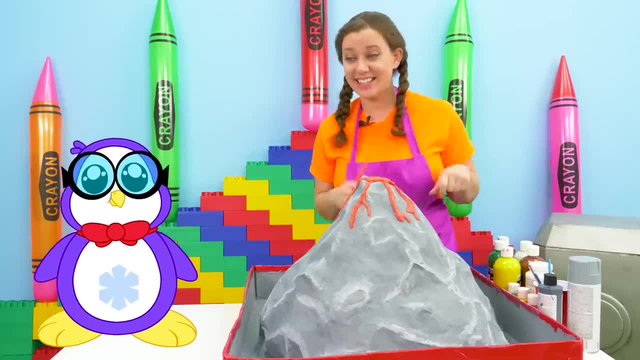 just finished our volcano and what do you think about it? i think our volcano, you think about it. i think our volcano, you think about it. i think our volcano is complete. looks like the real deal is complete. looks like the real deal is complete. looks like the real deal, huh. 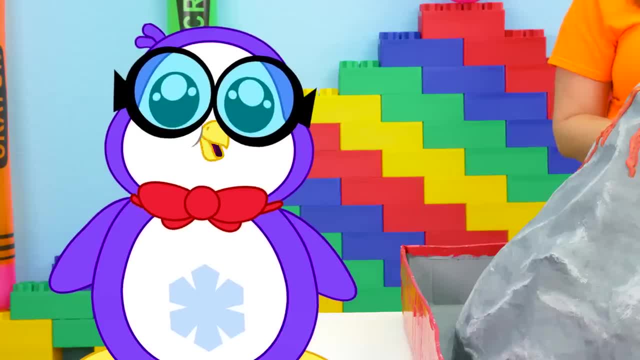 huh huh. looks like the one i saw earlier. looks like the one i saw earlier. looks like the one i saw earlier. let's teleport it to ryan. let's teleport it to ryan. let's teleport it to ryan. yay, the last thing we have to do is to. 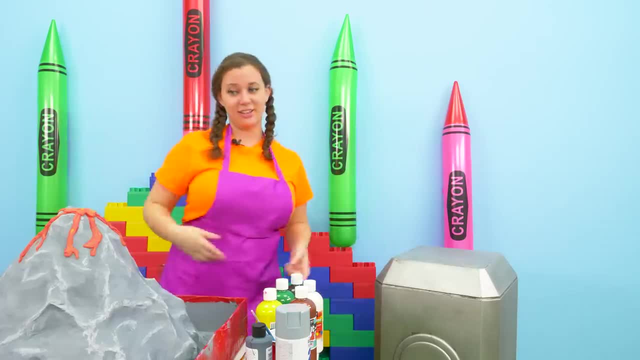 yay, the last thing we have to do is to yay. the last thing we have to do is to get this on to our teleportator potato, get this on to our teleportator potato, get this on to our teleportator potato. so let's just lift this guy. so let's just lift this guy. so let's just lift this guy. i'm just kidding, it's paper mache, it's. i'm just kidding, it's paper mache, it's. i'm just kidding, it's paper mache, it's really lightweight, really lightweight. 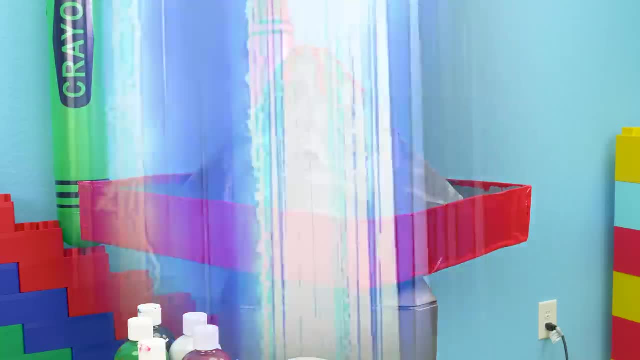 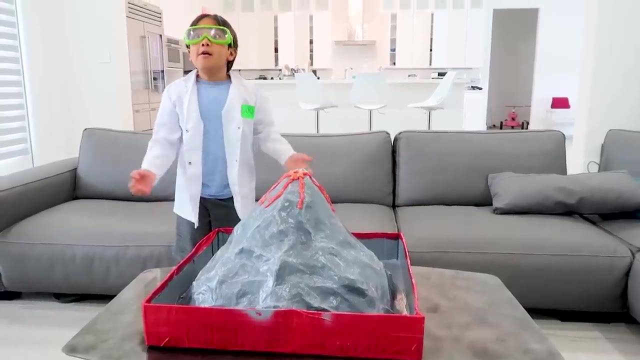 really lightweight. and off to ryan, we go. and off to ryan, we go. and off to ryan, we go. goodbye volcano, goodbye volcano, goodbye volcano. have fun ryan, wow, have fun ryan, wow, have fun ryan. wow, thank you so much, peck for this paper. 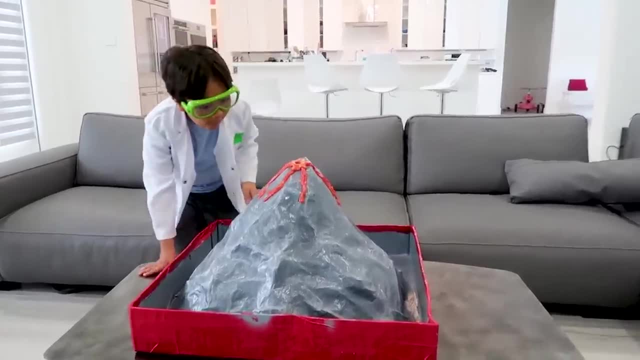 thank you so much, peck for this paper. thank you so much peck for this paper. volcano- it's so cool, super cool volcano. it's so cool, super cool volcano. it's so cool, super cool. i'm gonna bring it outside and then i'm. i'm gonna bring it outside and then i'm. 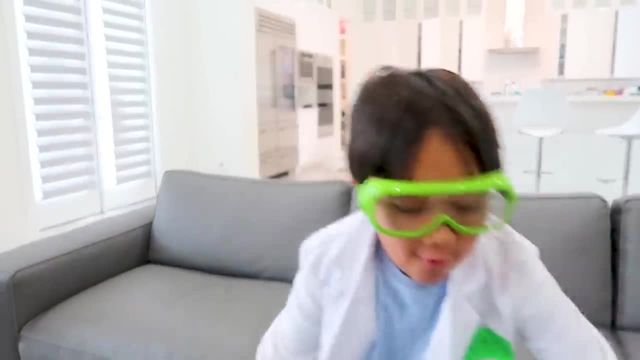 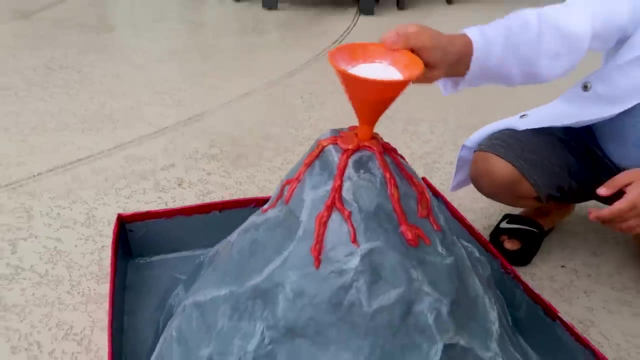 i'm gonna bring it outside and then i'm going to going to going to erupt it. let's go erupt it. let's go erupt it. let's go. first thing baking soda, first thing baking soda, first thing baking soda. cool, okay guys. so let's pour in the vinegar. 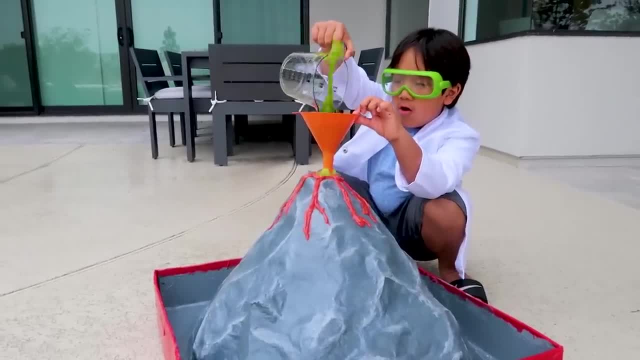 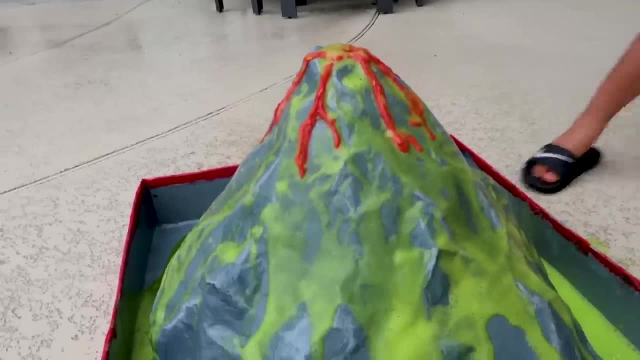 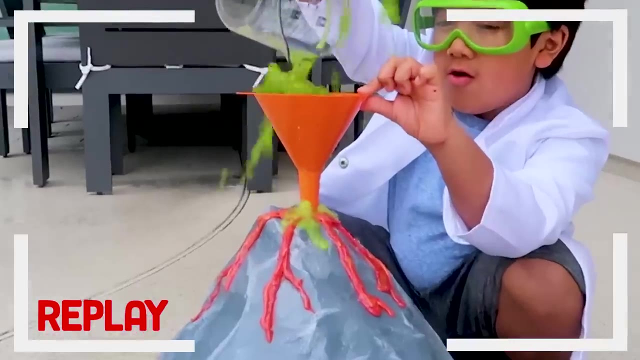 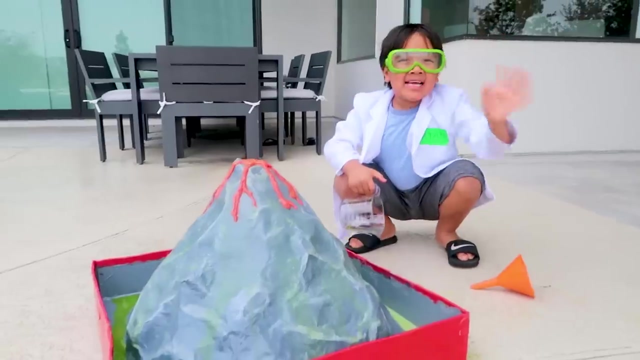 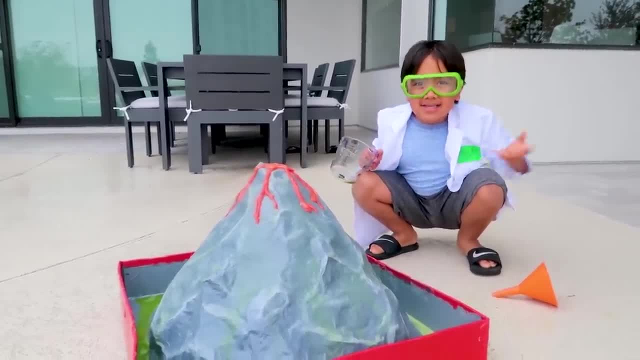 bye guys. thank you for watching our cool science experiment video with volcanoes. science experiment video with volcanoes. science experiment video with volcanoes. bye, remember, always stay happy and rise. bye, remember, always stay happy and rise by. remember, always stay happy and rise up, up, up, bye. bye, bye, bye, bye, bye.